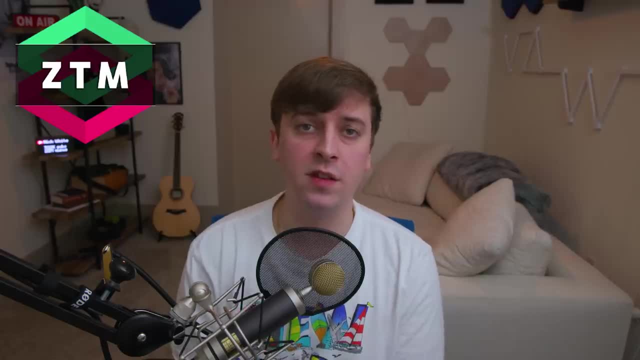 the tech industry And it's a really fitting sponsor for this video, because it's a really important one, because the founder of Zero to Mastery is also a self-taught programmer. They have over 50 courses and over 10,000 lessons in a bunch of different categories. Zero to Mastery. 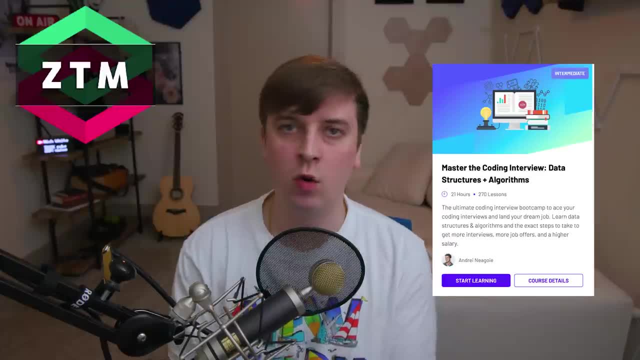 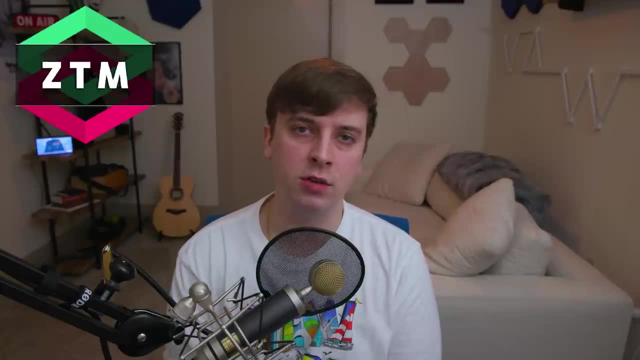 has courses for every step of your career, whether you're a beginner learning how to code, or whether you're a programmer trying to get a job, or whether you're a working professional and you just want to advance your skill set. They have world-class instructors and over a million students have. 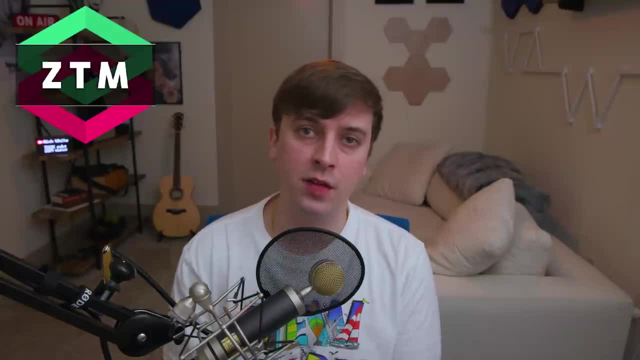 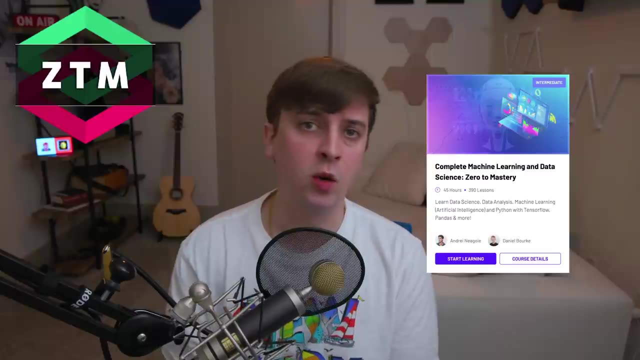 enrolled or graduated from their courses With over a thousand hours of content, and they're adding new courses all the time. So there's tons of content, whether you want to be a web developer or do cyber security, or do machine learning or web 3, or heck, even if you want to work on your. 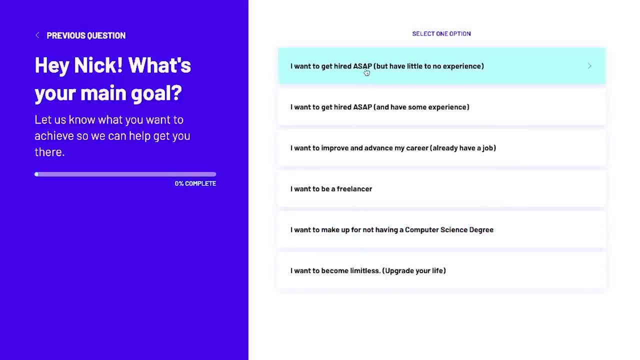 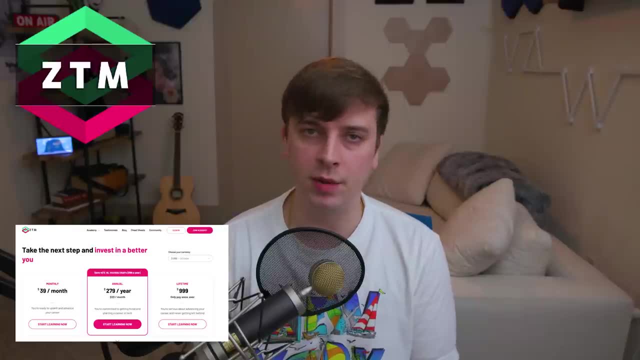 soft skills, And one of the coolest things they do is they have a career path quiz and, based on your current skill set and career goals, they recommend the perfect path of learning for you. They have monthly, annual and lifetime memberships and a ton of people use it and I think it's. 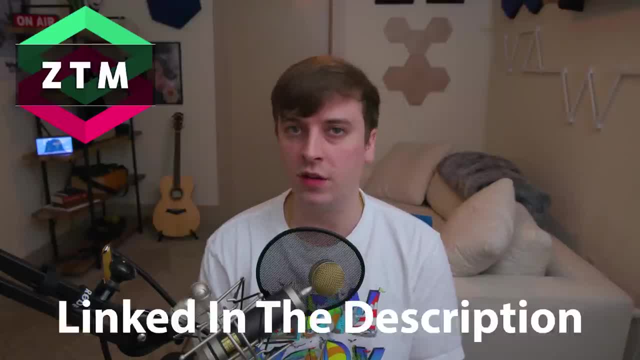 totally worth it. So if you guys are interested, definitely go into the description of this video, click the link and check it out. It's an awesome platform. Thank you for sponsoring this video. Zero to Mastery. and now let's get back to my opinions on self-taught. 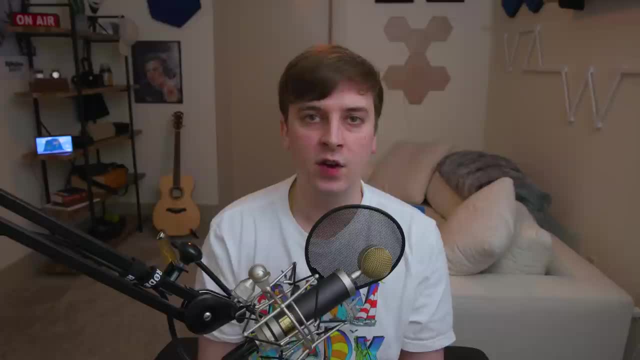 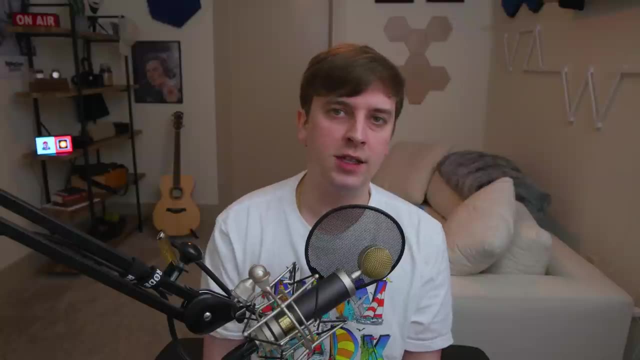 All right. so, coming from a traditional education background, my advice has always been: is college great? Yes, Do you need it? Absolutely not Now. of course, that's a little bit of a generalization, because there are programming jobs out there that do require a college degree When it comes. 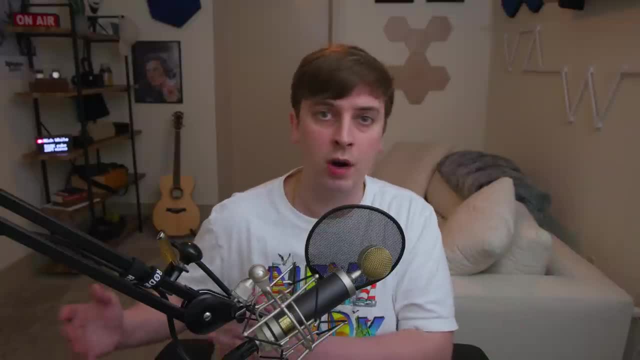 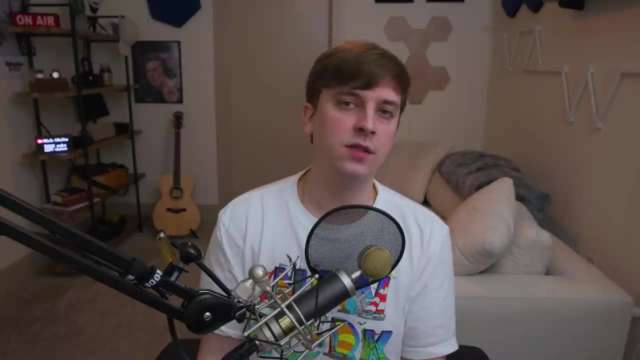 to advice on this, like: should you go the traditional education route versus self-taught programming route? it is really specific to you as a person, But since this is YouTube and I'm speaking to a lot of you here, I'm going to generalize and say that most programming jobs nowadays 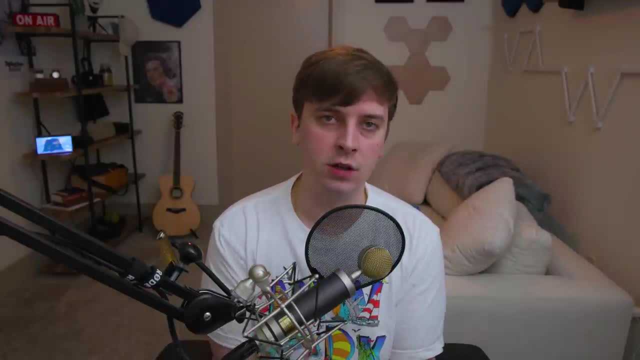 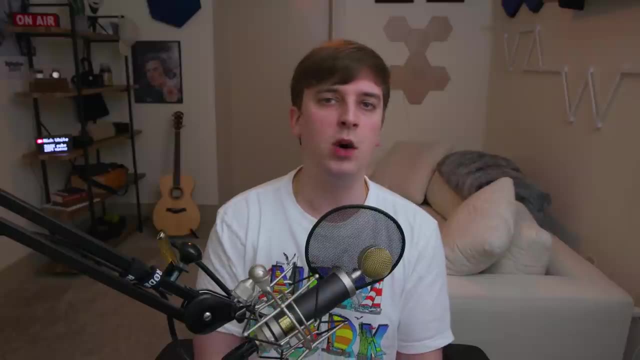 do not require a college degree. Over the past few years, people have started to place a lot of value on self-learning and since everybody moved to online and people have developed all these resources and courses, people understand how easy it is to self-learn and there's absolutely no way. 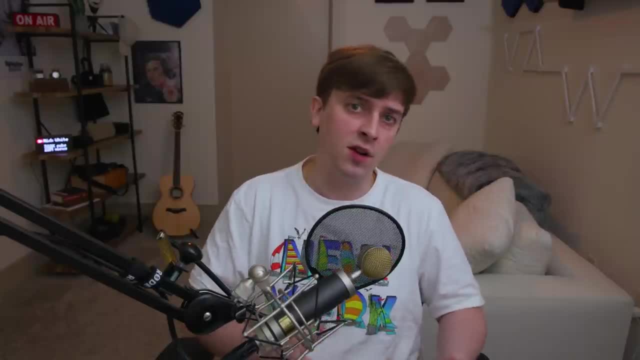 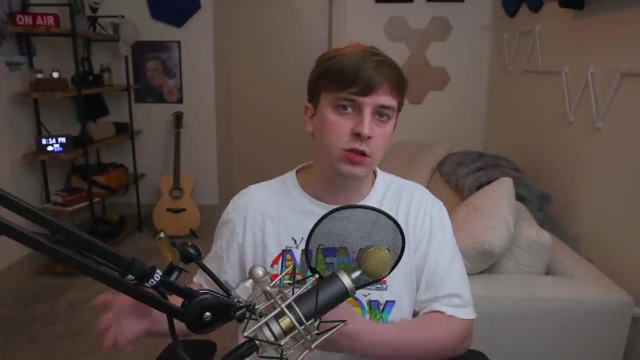 that anybody can say nowadays that a traditional education is necessarily more valuable than a self-taught education. The same information that you will be learning in traditional education you can teach yourself. That information is out there for everybody to learn. It's more dependent on you. 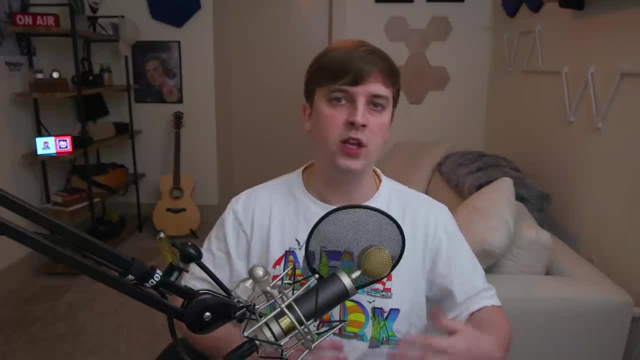 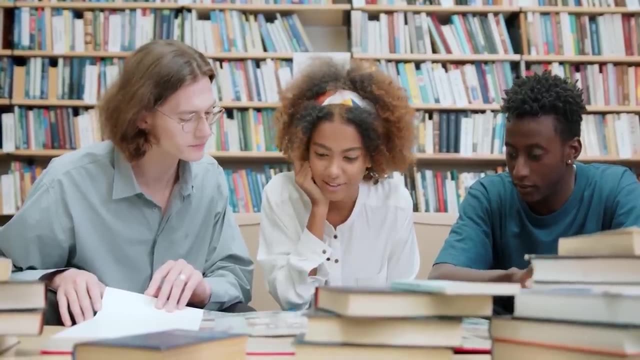 as a person and what you're learning is what you're learning, and what you're learning is what you're learning and what environment you want to put yourself into so that you can learn this stuff in the best way possible. College is great, right? you get to learn alongside peers and develop your 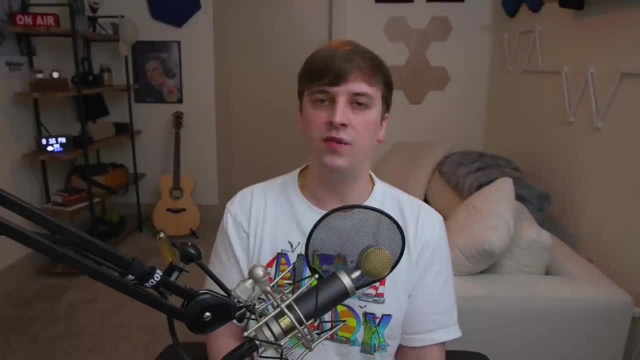 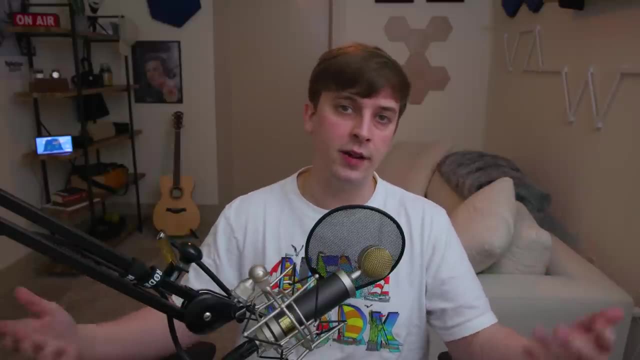 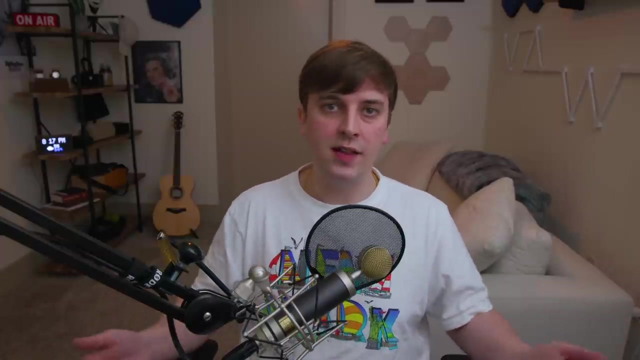 skills and learn from your peers and instructors who have different knowledge and different things, and you get face-to-face interaction with people, which makes communicating really easy for learning and retaining all this information. However, this doesn't necessarily mean it's the best environment for learning. First of all, it's tough to generally say that college computer science is a great thing. 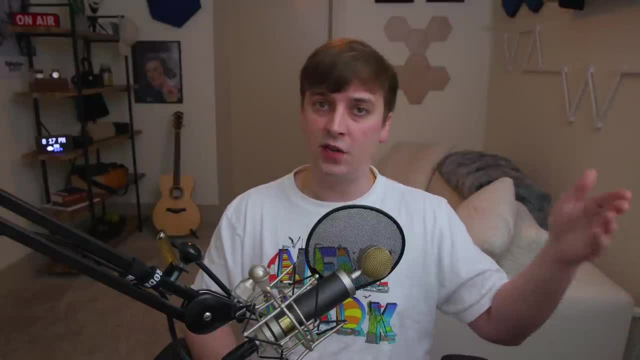 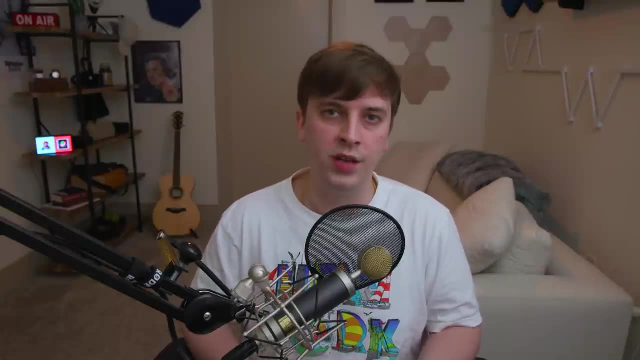 to go into considering every computer science program at every different university or college is completely different. The instructors will be different, the people will be different, the environment will be different, the material will be different. and when you're enrolled in a program in college and you're having a tough time learning from an instructor, the way to change your 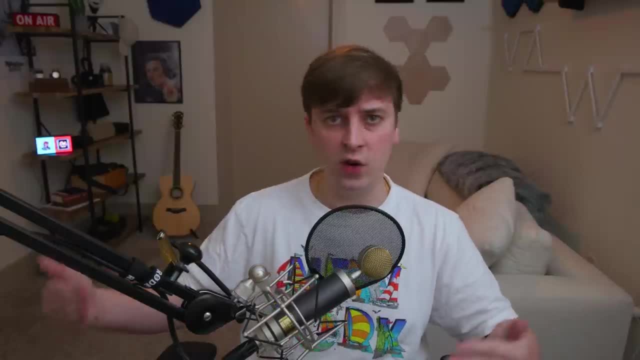 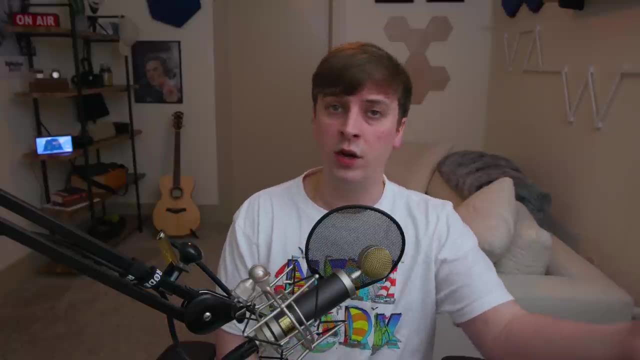 instructor would be to drop the class or switch the class or maybe switch universities all together into a different program, whereas if you're self-teaching and you're trying to learn something and you have a certain resource that isn't doing it for you, you could switch, take a different course. 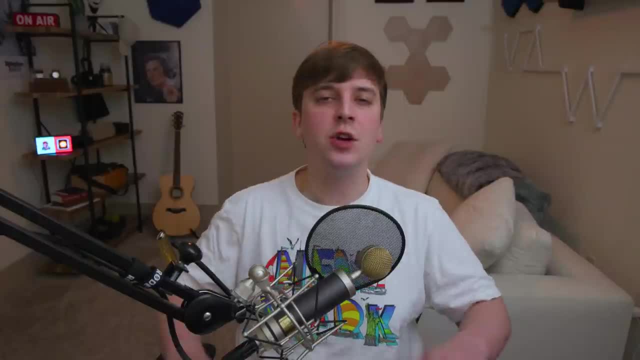 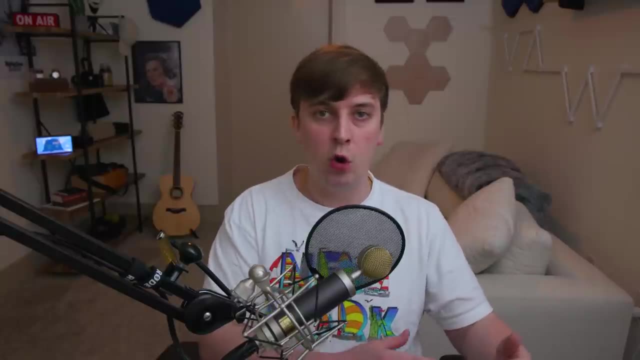 from an instructor and maybe learn it from someone else that easily. I just don't necessarily think there's any right way for you to learn. Just because you went to college doesn't necessarily mean that you're going to know more or be any better of a programmer than somebody who's self. 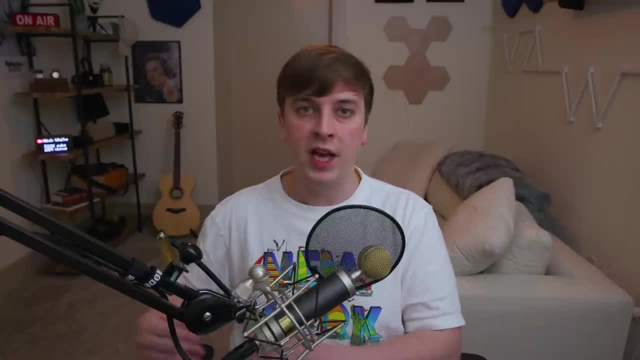 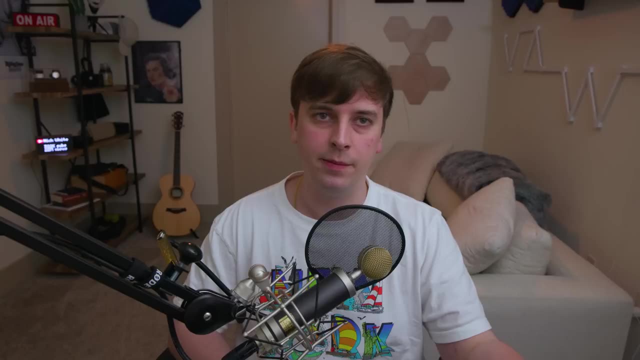 taught, and just because you're self-taught doesn't mean you know any better or are going to be any better of a programmer than somebody that went to college. Because of societal conventions, people put a lot of value on the college degree. However, I don't know about you guys, but when I was in 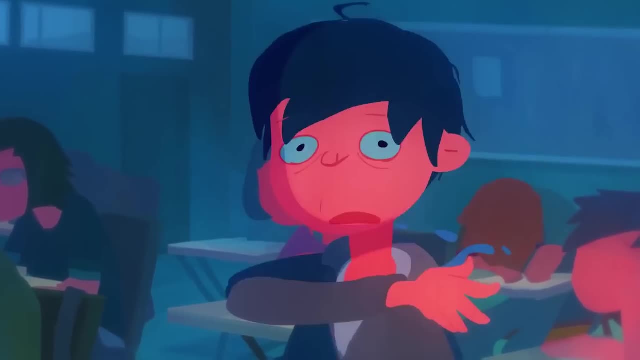 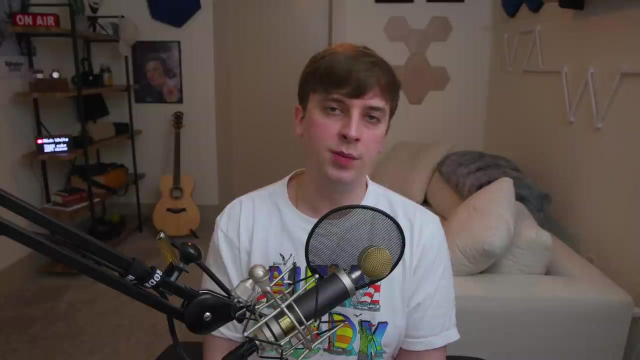 college I remember there were a lot of people partying, sleeping in class, skipping class and people cheating. But when it comes to self-taught programming, there's also flaws there. Some people have a tough time learning on their own, whether it's because they can't commit to a 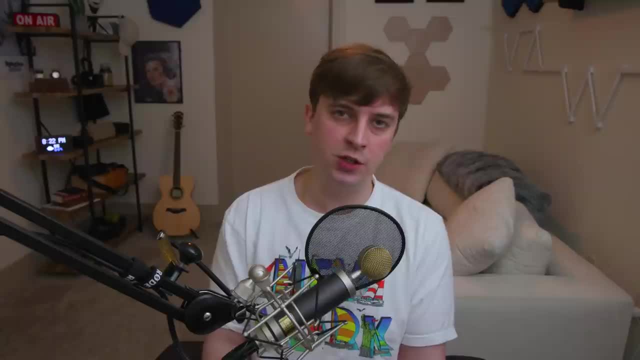 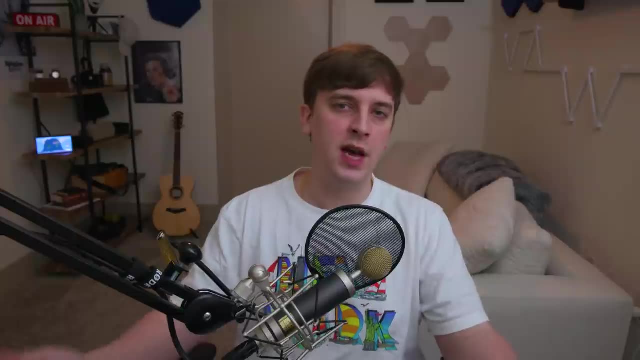 schedule of learning and practicing every single day, or because they have comprehension issues and they're the type of learner that needs to ask questions and have face-to-face communication with somebody to actually learn. Generally, to me it doesn't really matter which way you choose to learn, whether you want to go traditional education or self-taught programmer, it doesn't. 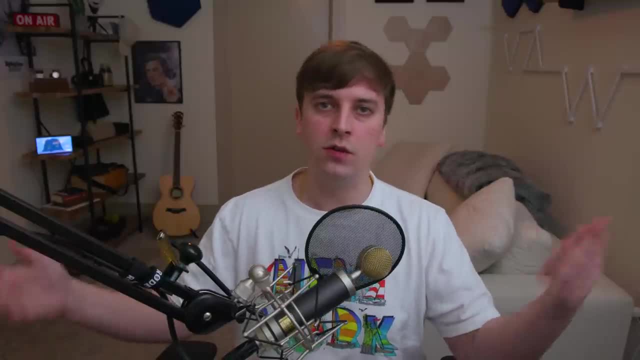 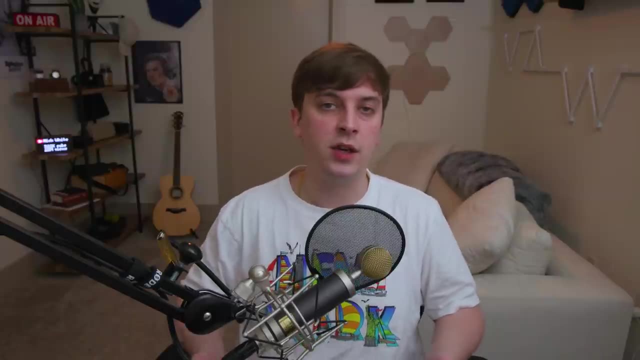 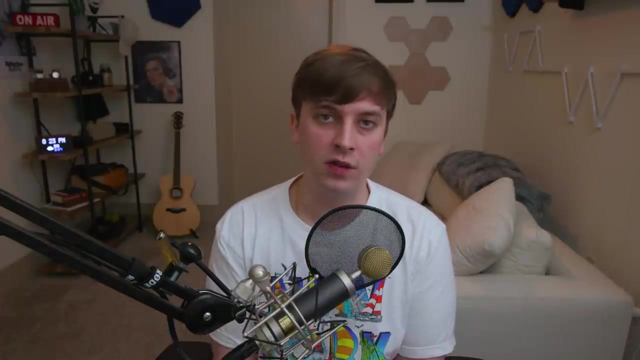 really matter. All that matters is that you learn and develop your skills right until it comes to the actual commitment. Now, education is extremely valuable and it's actually considered investing in yourself. There's been a charge for education for forever, and valuable educational resources can become very pricey, but it's up to you to not make bad financial decisions. This is extremely 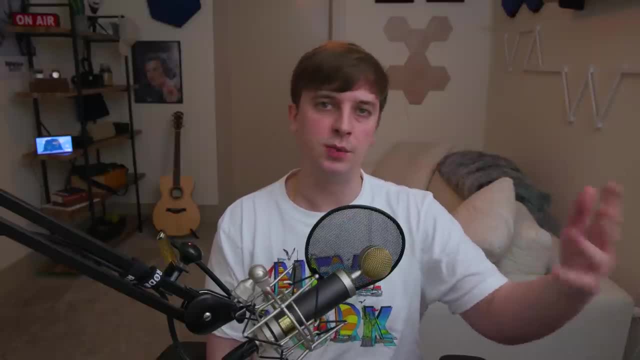 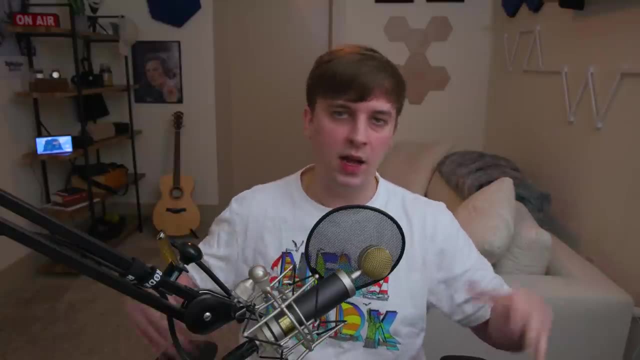 important to understand, because a lot of people just look to programmers and people that have software engineering roles and see how much money they make and just think: I want to do that, let me get to there. no matter what it takes, I'll do whatever I'll pay the most money for. 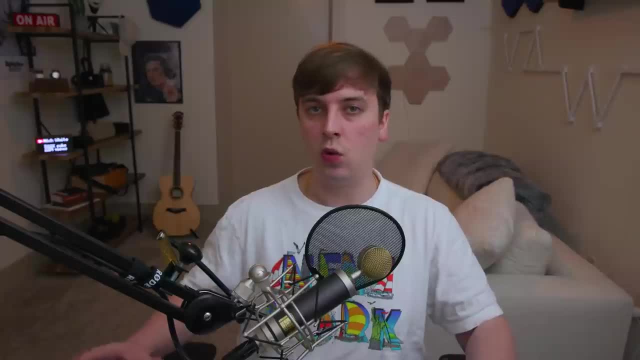 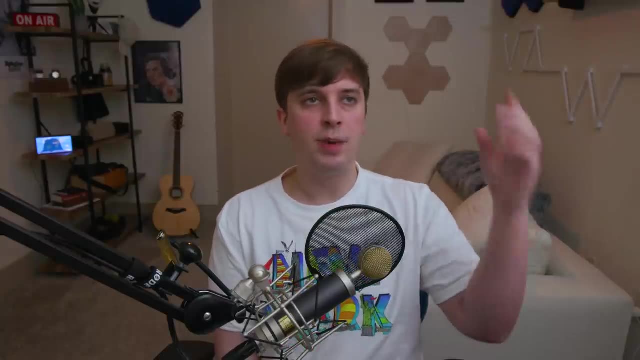 education, and just just get me to that point. But you shouldn't just automatically equate an expensive education to a valuable education, and thinking of an education like an investment is really important. right, you could buy a really expensive stock, but maybe it's actually not that. 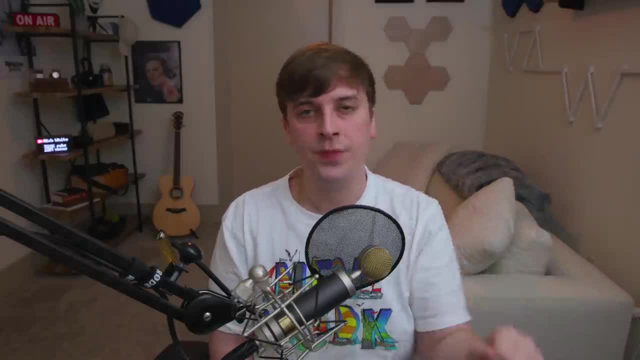 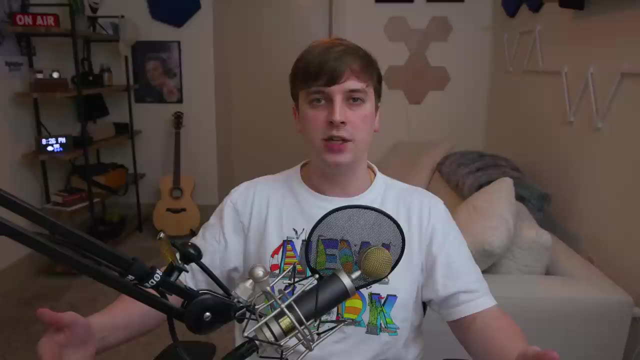 valuable and over time you're going to lose money for investing in that stock. Well, when you invest in your education, you want a valuable education that is going to have a return on that investment. so you might pay for your education, but it makes you a lot of money. in the long run you get a. 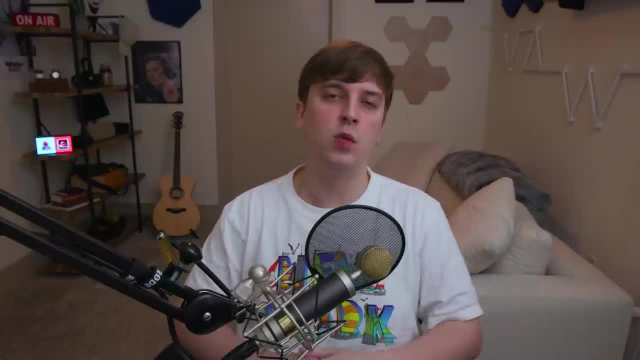 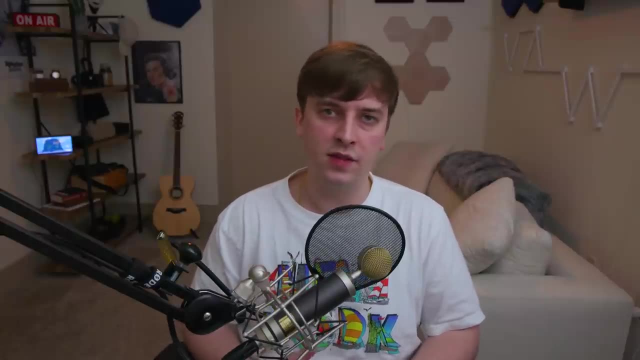 successful career out of it, and it's totally worth it. You may not, however, want to pay for an expensive education and then not make a lot of money from it, and this happens to a ton of people when they go to a really expensive school and they think it's. 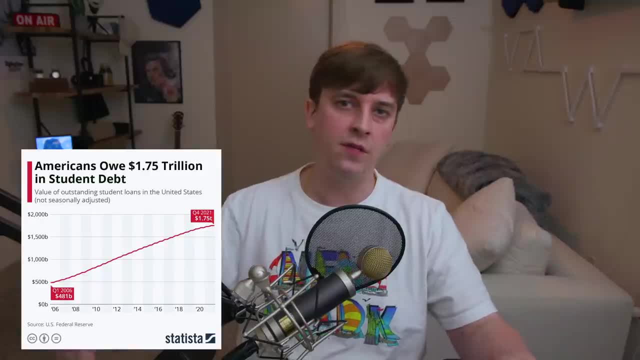 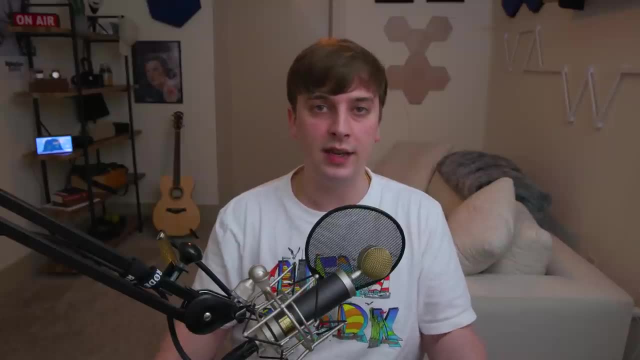 going to be a really great life decision, but they don't actually learn that much and develop the skill set they need to have a really successful career and get that return on investment. Instead, you might be stuck with a ton of student debt and no job. This could also happen at something. 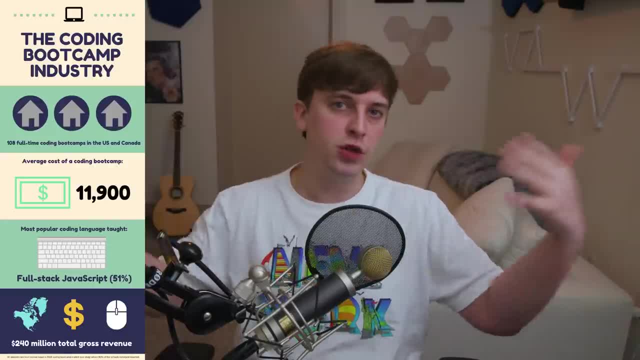 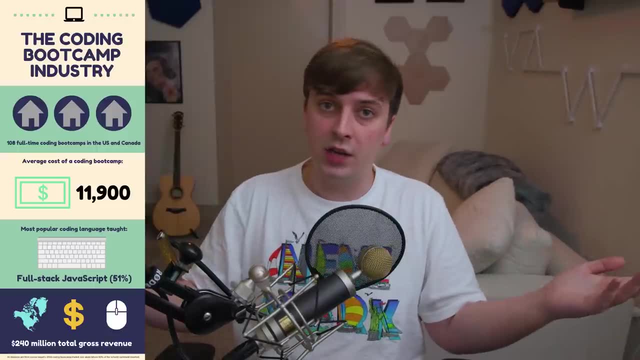 like a boot camp that's extremely expensive, that advertises that you should be able to get a job after nine weeks, but maybe they don't guarantee it right and you pay all of this money for the boot camp. but what if you don't get the job after? So, unless you're completely fine with wasting? 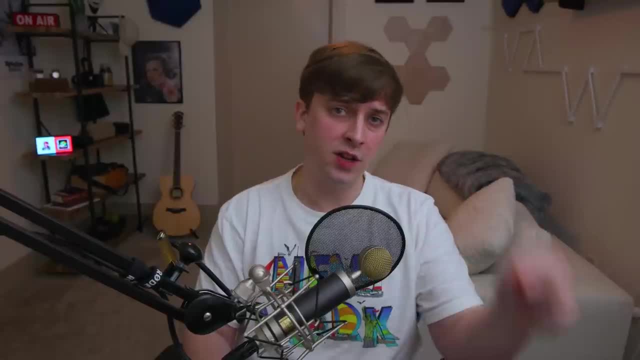 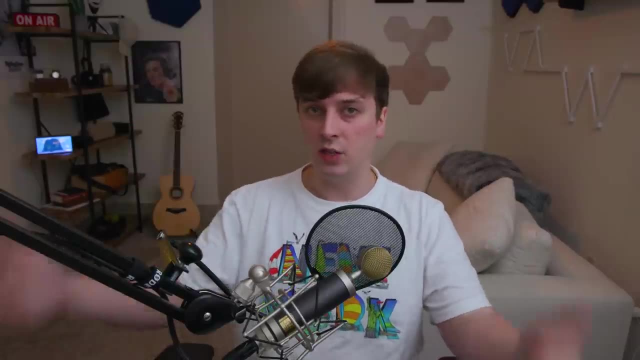 money and going into debt. you need to be extremely careful when you're considering the investment for your education. Make sure that you fully understand what you're getting yourself into and what you're going to learn from this education and what you're going to do with those skills afterwards to get 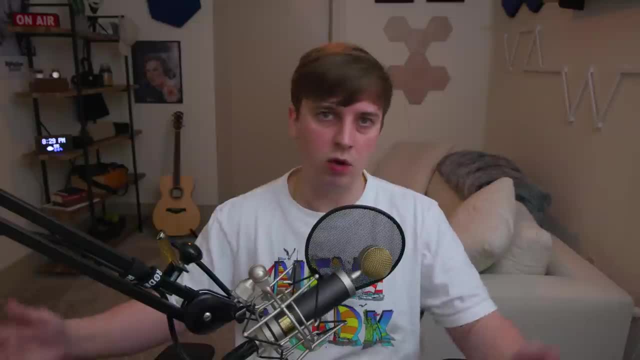 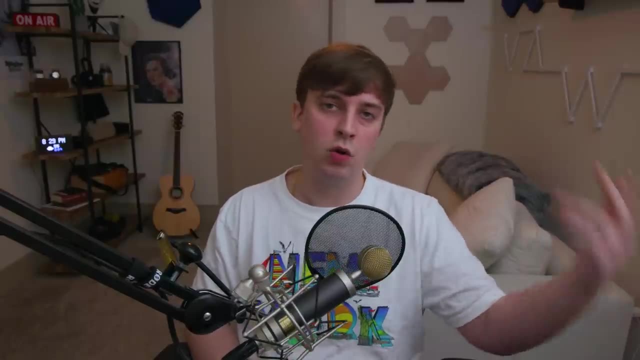 that return on investment. So those are my opinions and advice on self-taught programming versus traditional education. but since I'm not actually a self-taught programmer, I'm now going to throw it at the programming YouTuber. So let's talk about ways that you could learn how to code as a self-taught. 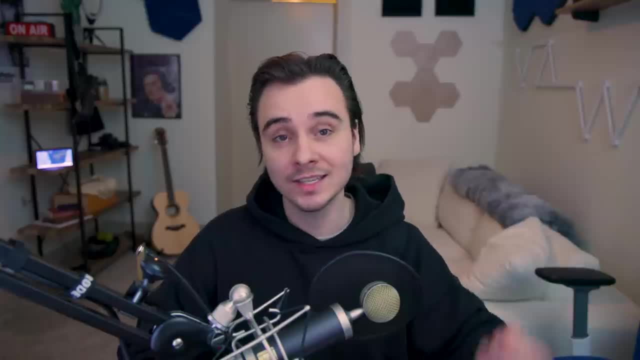 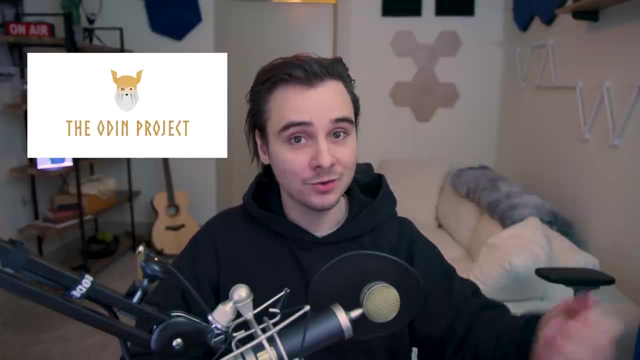 programmer. Now there's a lot of great material out there online and a lot of it is actually free Resources that I've heard a lot of good things about are Free Code Camp, The Odin Project, and then there's a great lecture series by Harvard on YouTube called CS50.. You may have heard of it. 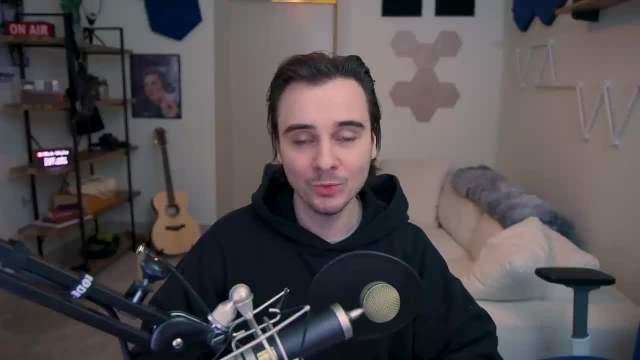 before, but I think it's important to realize when learning how to code. it's not a one-size-fits-all solution. You can start with Free Code Camp, you could start with The Odin Project, or you could start with the CS50 course, and maybe that just doesn't work out for you. I originally wanted to 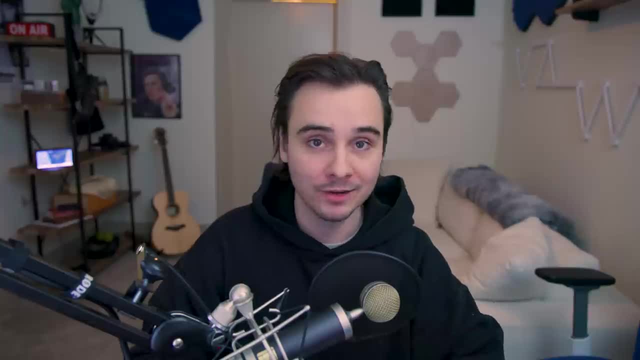 start learning how to code because I wanted to make mods for the game Minecraft and when I started I didn't have a solid structure. I didn't have a thing like The Odin Project or Free Code Camp to guide me. I watched a couple YouTube tutorials to get my IDE set up in Java, and then I watched a 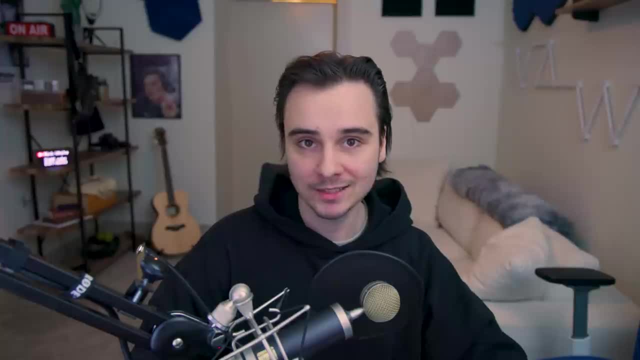 couple tutorials on how to make Minecraft mods, and I think another really important thing to understand is that when you are first learning how to code and you're watching tutorials, the information isn't going to click right away. I remember I was watching these tutorials and how to build these mods and I was typing out: 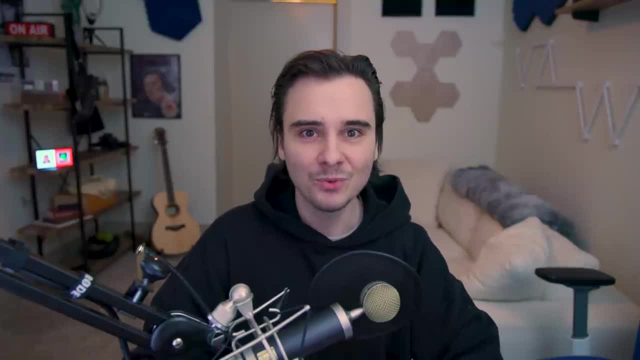 the functions and making the classes and I didn't understand really how it was working. I was kind of just copying the code and praying that it would run. But the thing is, if you do that consistently enough and you do that for a long period of time, things just start to click And I think the best 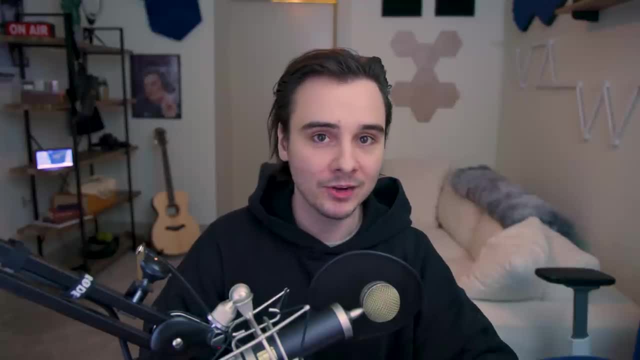 advice that I could give you is that if you want to get better at learning how to code as a programmer, is you got to keep exploring resources. Figure out resources that work well for you, but just don't stop coding. As cliche as that sounds, you really just got to keep coding. You got to. 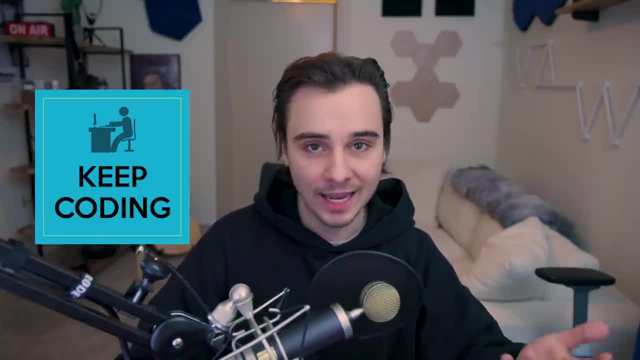 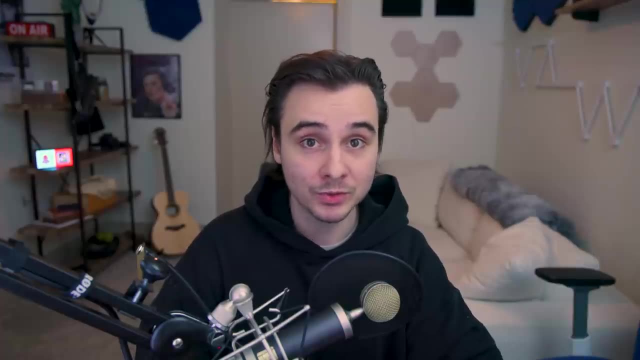 keep banging your head against the wall, You got to keep googling to find answers to your bugs, so on and so forth. And once you start getting down the basics, you won't have to rely on a tutorial to actually code. You'll eventually be able to make your own projects without a tutorial, and that is. 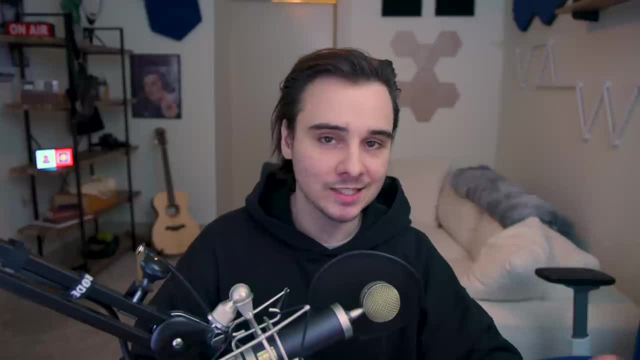 something I highly encourage you to do: Come up with a tutorial and I'll see you in the next video. Bye, project idea. it doesn't really matter what the project idea is. honestly, I think a good place to start would be something like a Twitter clone or a YouTube clone or something of that nature. just 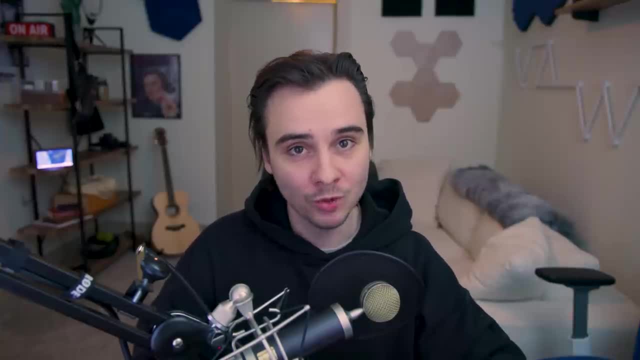 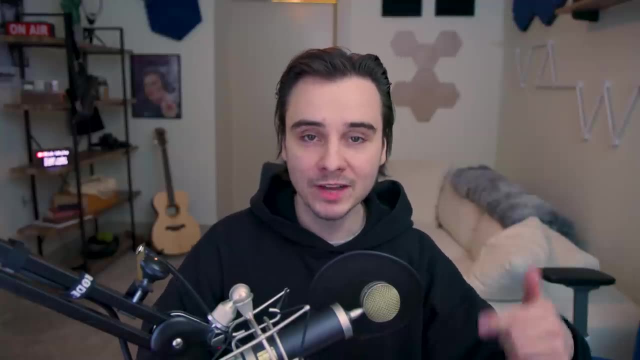 come up with an idea- doesn't have to be unique, but don't follow a tutorial when you're writing it. start building the project, get stuck, use Google to help guide you, so on and so forth. eventually you do that enough you'll build your own personal projects. maybe you'll start building. 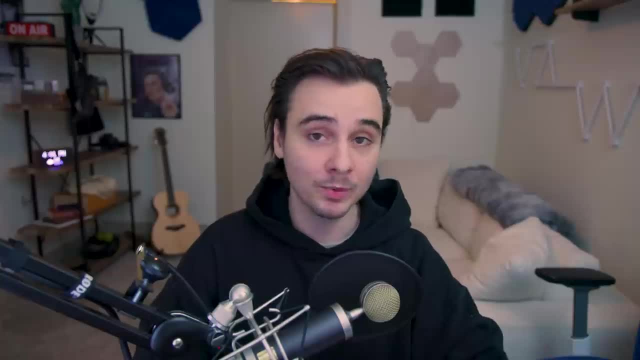 a portfolio. maybe you host that with GitHub or maybe you build a website portfolio displaying all your work. but don't expect to go from first starting to learn how to code to building these cool projects and making a portfolio overnight. it can take weeks, months, sometimes even years to get. 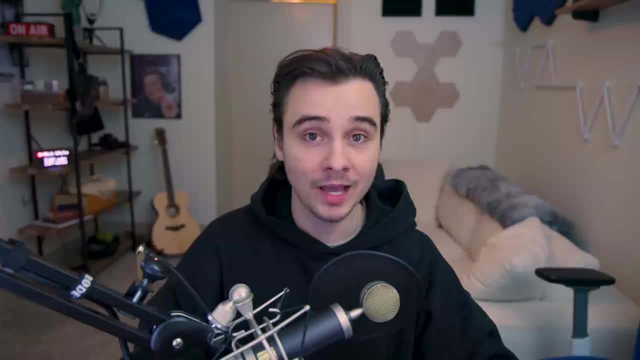 to that level once you build your developer portfolio. that's when the exciting part happens and that's when you can start applying for jobs. but don't be too discouraged. if you start applying for jobs and you don't hear back right away. you can oftentimes take hundreds of applications. 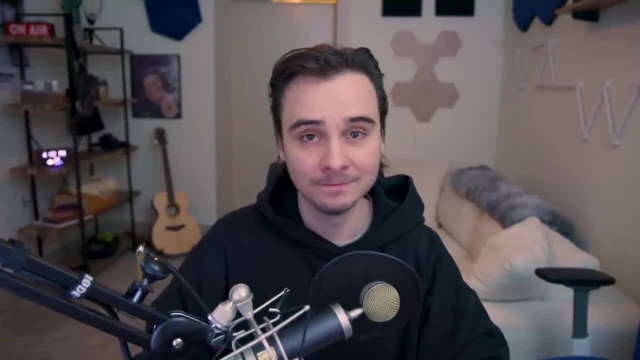 but the important thing is to be consistent when you apply. another great piece of advice that I give out is that building your network as a self-taught programmer is important, because oftentimes it's not about what you know, it's about who you know when it comes to getting a. 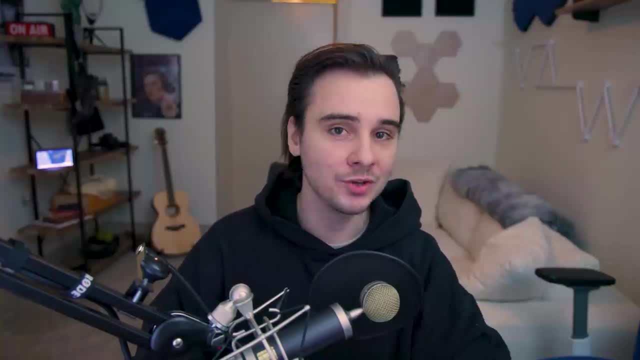 job. there's many different ways you can Network in this digital age. you can join Discord groups, you can just find people online, or you can meet up with people in real life and go to tech conferences, talk to the recruiters there, get their business cards, get their emails and then reach out to them like that. so build your network. stay consistent when applying. 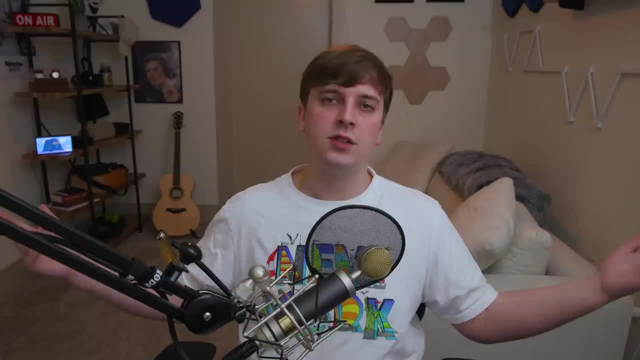 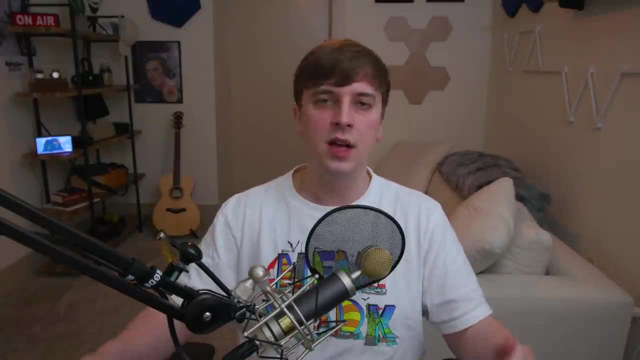 for jobs but also stay consistent when learning how to code. all right, so that's pretty much it, guys. I was just making this video to kind of cover on some of these very big general coding YouTuber topics. this is one of the ones I haven't really talked about in depth yet. I know a lot of people. 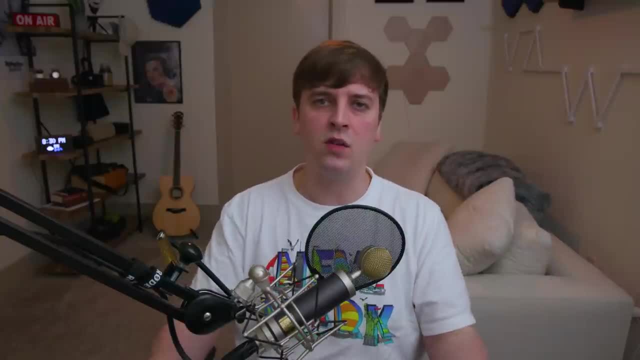 are learning from different ages and backgrounds and you all have different crazy stories about traditional education, self-taught programming, getting hired in the tech industry. maybe didn't get hired. I'd love to see those in the comments below and I'll see you guys in the next video. 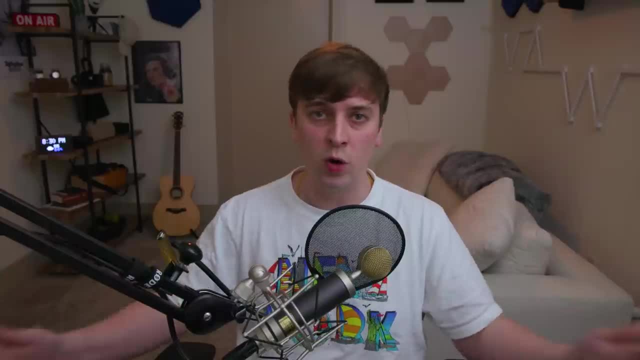 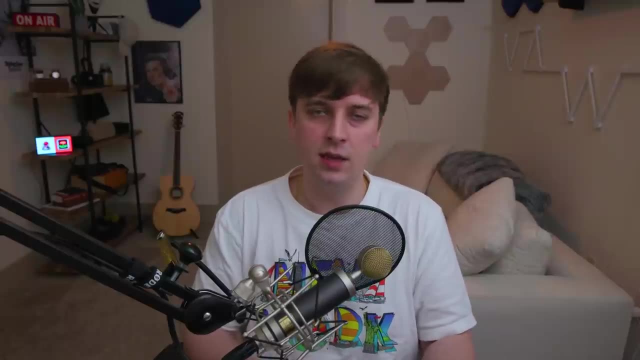 comments below. I always want to read and see what's going on currently in the world, so please drop some comments so I can read from your stories. maybe you can educate me a little bit. if you enjoyed this video, please leave a like, subscribe to the channel and if you want to, 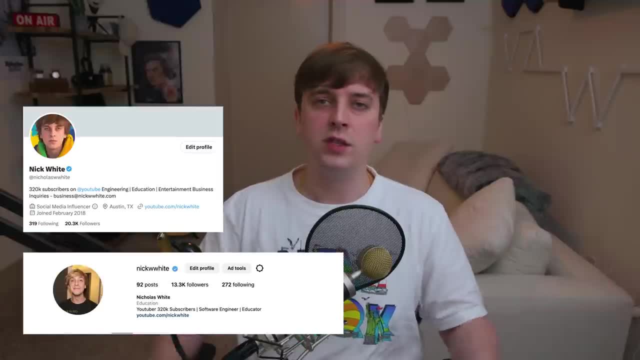 connect with me more personally: follow me on Instagram and Twitter. thank you guys for watching this video. as always, I appreciate all your support and see you guys, in the next one- peace.